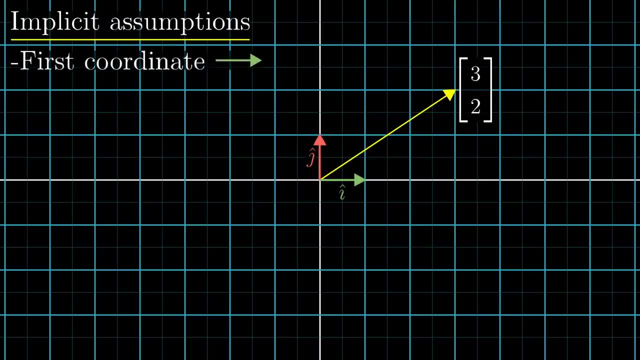 system, The fact that the first number indicates rightward motion, that the second one indicates upward motion, exactly how far a unit of distance is. all of that is tied up in the choice of i-hat and j-hat, as the vectors, which are scalar coordinates, are meant to actually scale Any 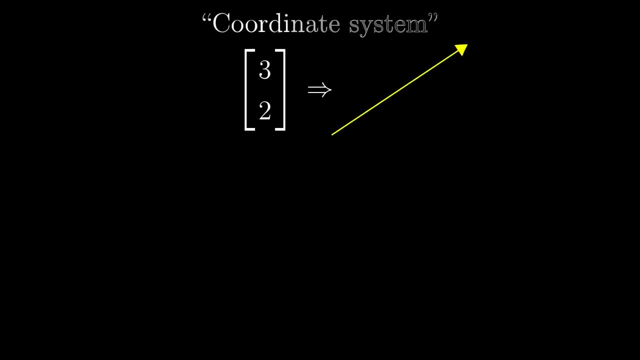 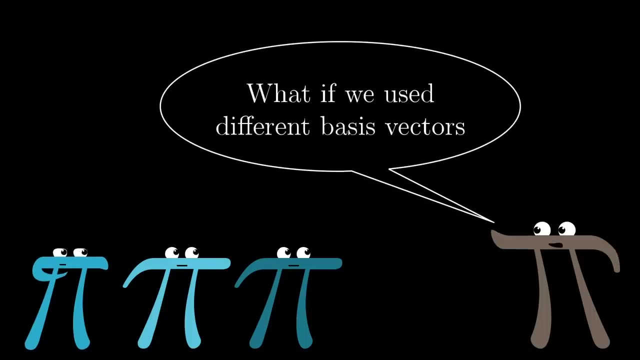 way to translate between vectors and sets of numbers is called a coordinate system, and the two special vectors, i-hat and j-hat, are called the basis vectors of our standard coordinate system. What I'd like to talk about here is the idea of using a different set of basis vectors. 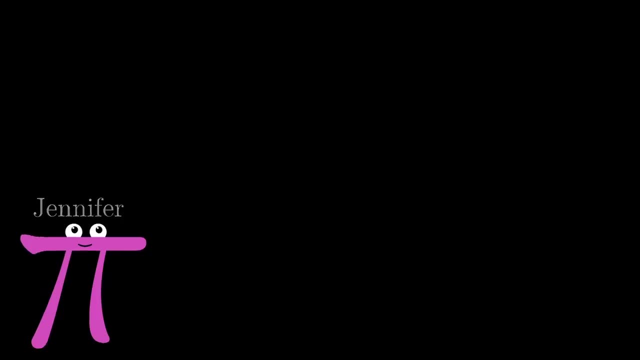 For example, let's say you have a friend, Jennifer, who uses a different set of basis vectors, which I'll call b1 and b2.. Her first basis vector, b1,, points up and to the right a little bit, and her second vector, b2,, points left and up. Now take another look at that. 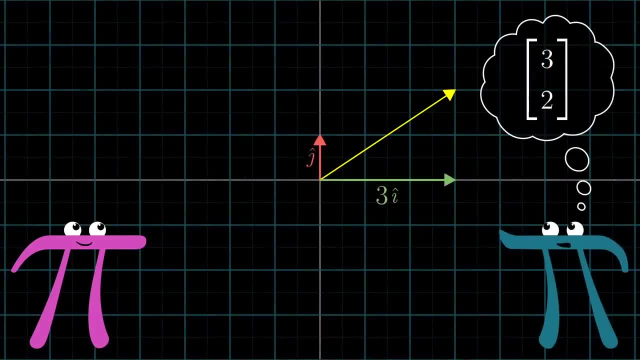 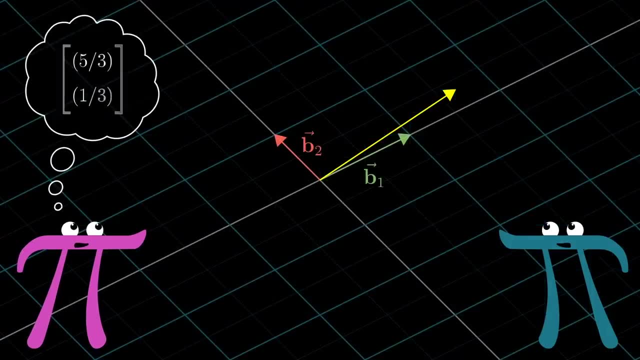 vector that I showed earlier, the one that you and I would describe using the coordinates, using our basis vectors i-hat and j-hat. Jennifer would actually describe this vector with the coordinates 5 thirds and 1 third. What this means is that 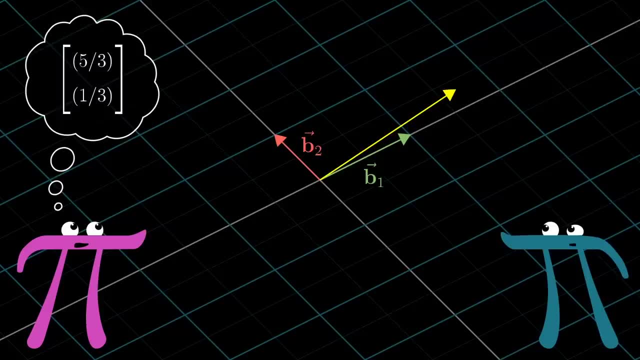 the particular way to get to that vector using her two basis vectors is to scale b1 by 5 thirds, scale b2 by 1 third, then add them both together. In a little bit I'll show you how you could have figured out those two numbers- 5 thirds and 1 third- In general. 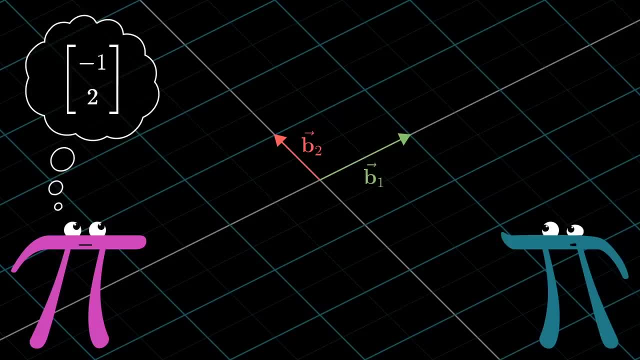 whenever Jennifer uses coordinates to describe a vector, she thinks of her first coordinate as scaling b1,, the second coordinate as scaling b2, and she adds the results. What she gets will typically be completely different from the vector that you and I would think of as 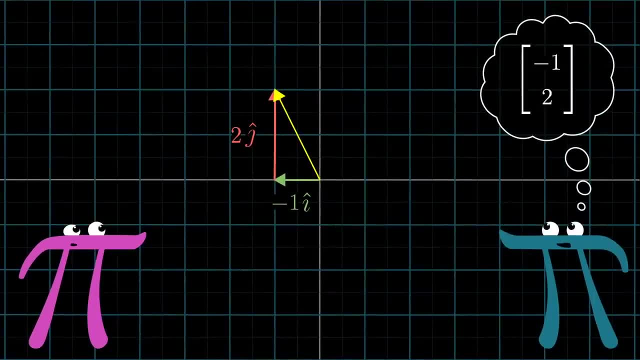 having those coordinates. To be a little more precise about the setup here, her first basis, vector b1, is something that we would describe with the coordinates, and her second basis, vector b2, is something that we would describe as, But it's important to realize from her perspective. 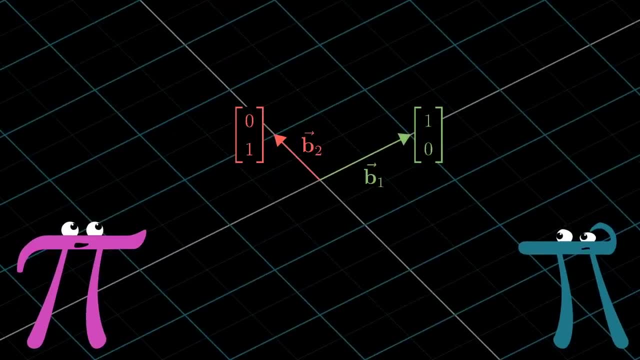 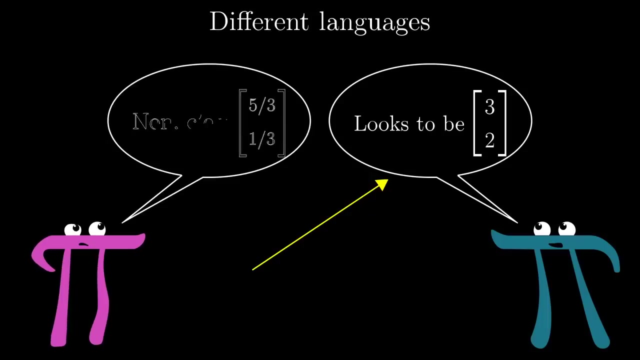 in her system. those vectors have coordinates. they are what define the meaning of the coordinates in her world. So, in effect, we're speaking different languages. We're all looking at the same vectors in space, but Jennifer uses different words and numbers. 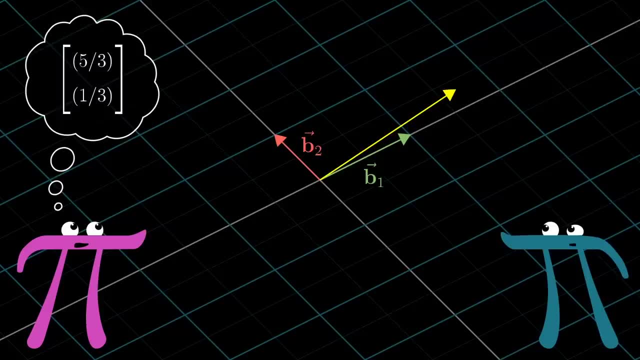 the particular way to get to that vector using her two basis vectors is to scale b1 by 5 thirds, scale b2 by 1 third, then add them both together. In a little bit I'll show you how you could have figured out those two numbers- 5 thirds and 1 third- In general. 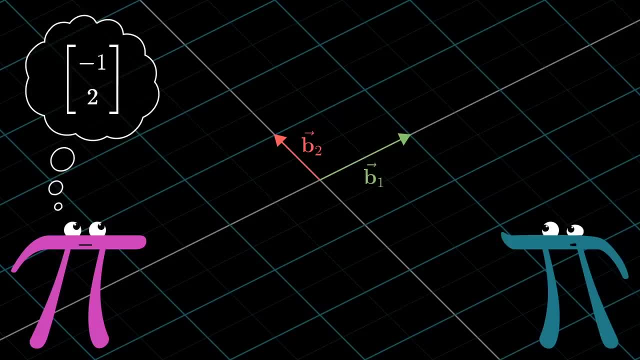 whenever Jennifer uses coordinates to describe a vector, she thinks of her first coordinate as scaling b1,, the second coordinate as scaling b2, and she adds the results. What she gets will typically be completely different from the vector that you and I would think of as 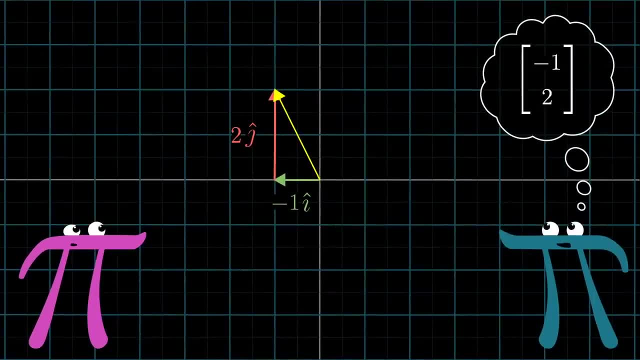 having those coordinates. To be a little more precise about the setup here, her first basis, vector b1, is something that we would describe with the coordinates, and her second basis, vector b2, is something that we would describe as, But it's important to realize from her perspective. 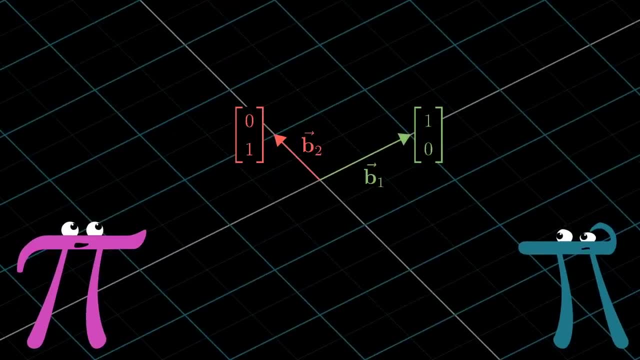 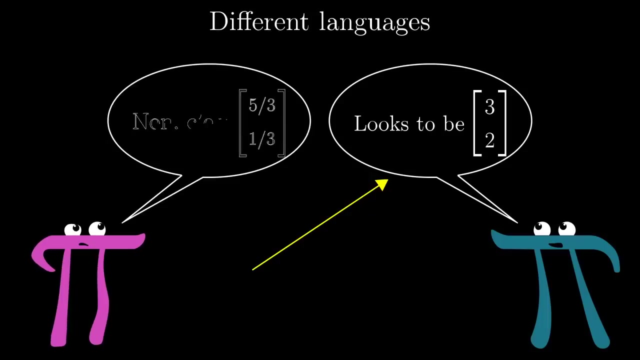 in her system. those vectors have coordinates. they are what define the meaning of the coordinates in her world. So, in effect, we're speaking different languages. We're all looking at the same vectors in space, but Jennifer uses different words and numbers. 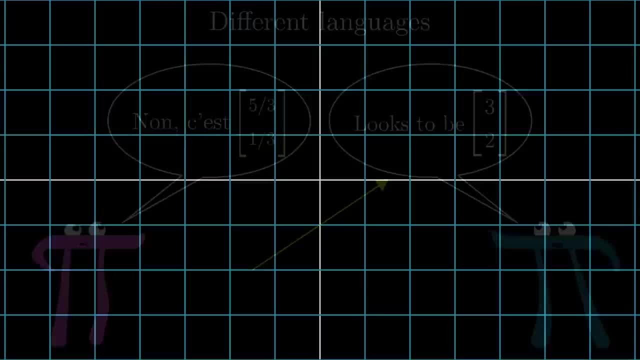 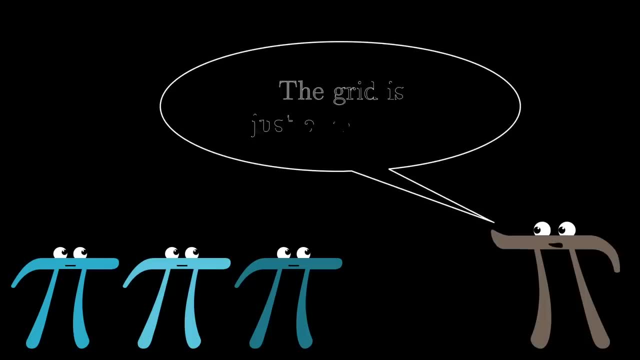 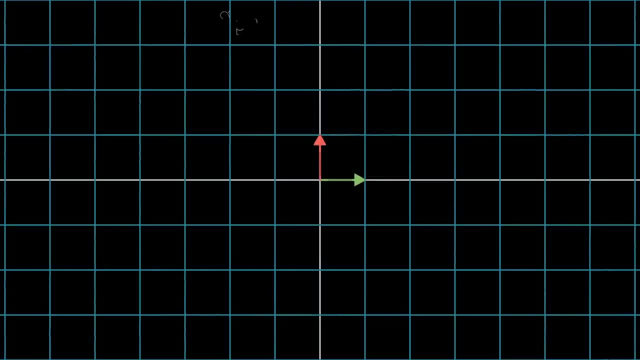 to describe them. Let me say a quick word about how I'm representing things here. When I animate 2D space, I typically use this square grid, But that grid is just a construct, a way to visualize our coordinate system, and so it depends on our choice of basis. 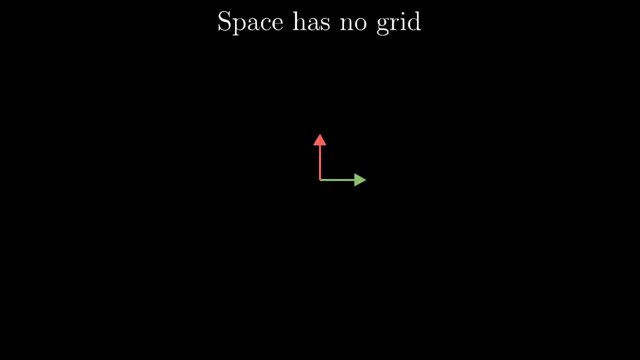 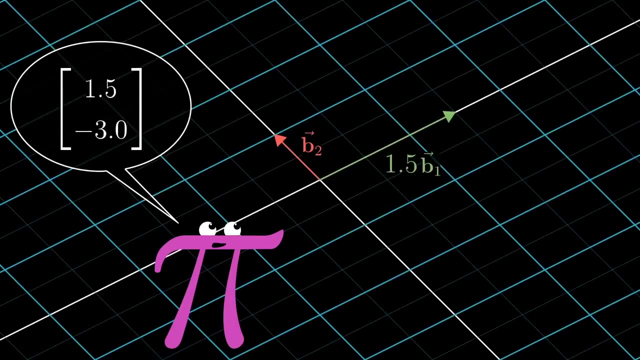 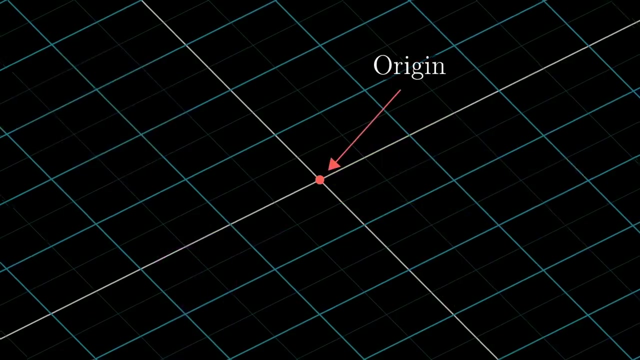 Space itself has no intrinsic grid. Jennifer might draw her own grid, which would be an equally made-up construct, meant as nothing more than a visual tool to help follow the meaning of her coordinates. Her origin, though, would actually line up with ours, since everybody. 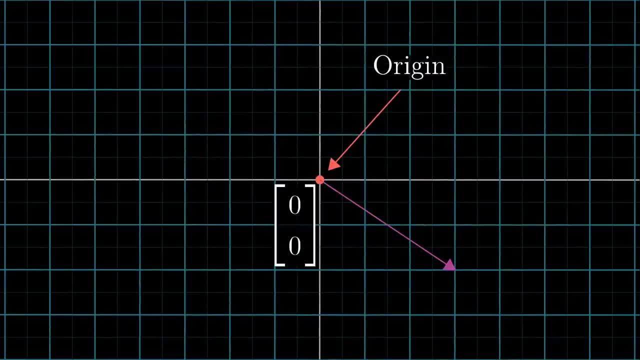 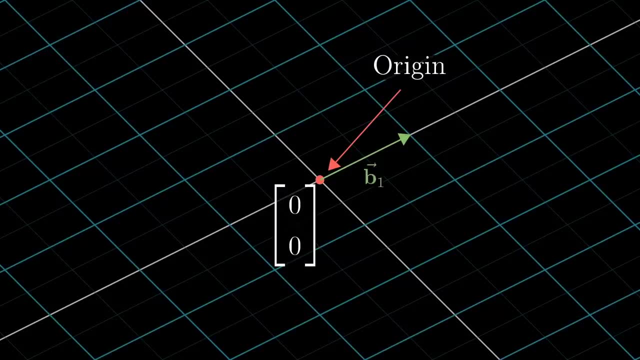 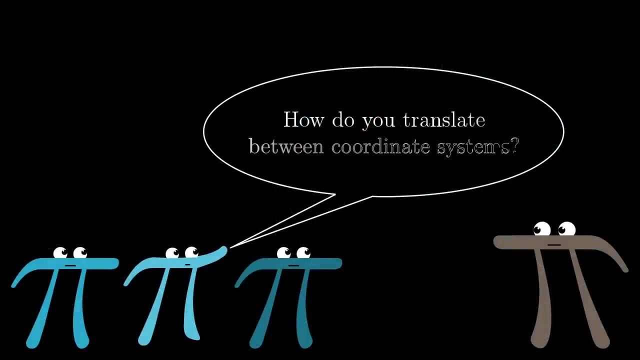 agrees on what the coordinates should mean. It's the thing that you get when you scale any vector by zero, But the direction of her axes and the spacing of her grid lines will be different depending on her choice of basis vectors. So, after all, this is set up. a pretty natural question to ask is how we translate between: 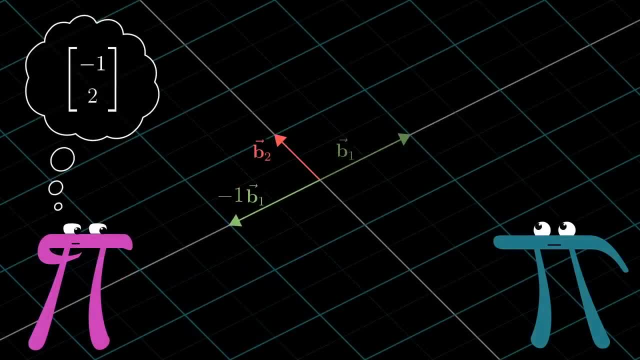 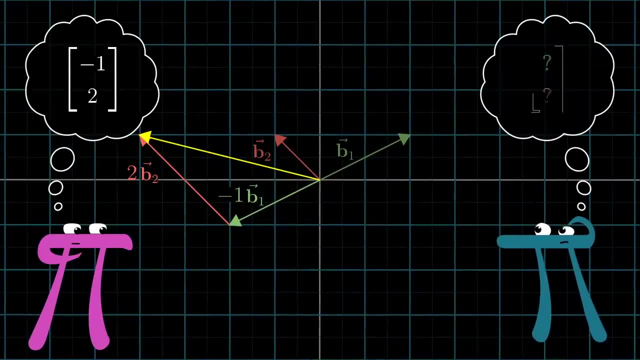 coordinate systems. If, for example, Jennifer describes a vector with coordinates, what would that be in our coordinate system? How do you translate that? Well, that's the question. How do you translate from her language to ours, Well, what her coordinates? 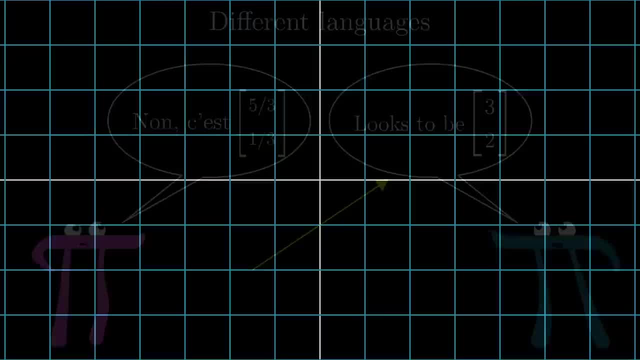 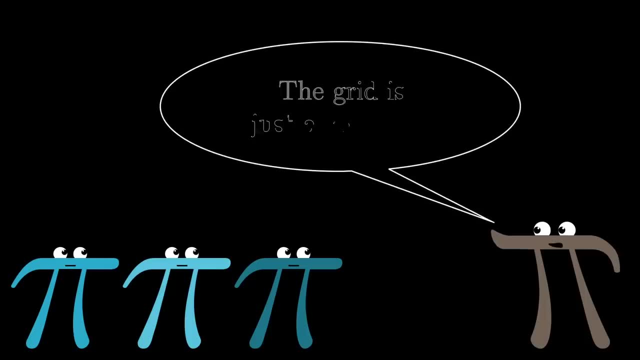 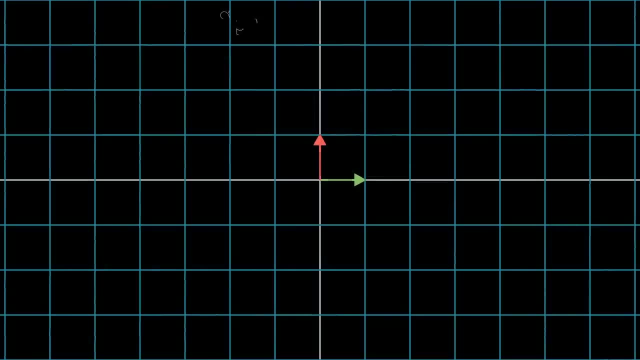 to describe them. Let me say a quick word about how I'm representing things here. When I animate 2D space, I typically use this square grid, But that grid is just a construct, a way to visualize our coordinate system, and so it depends on our choice of basis. 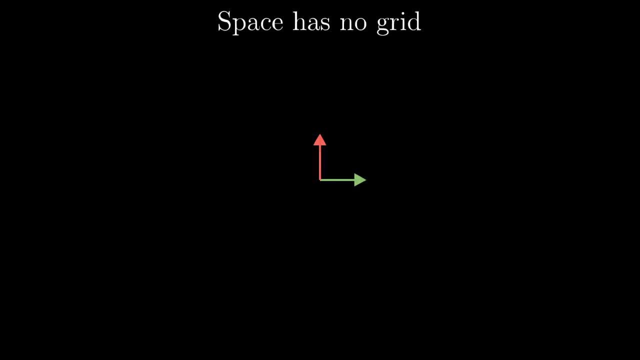 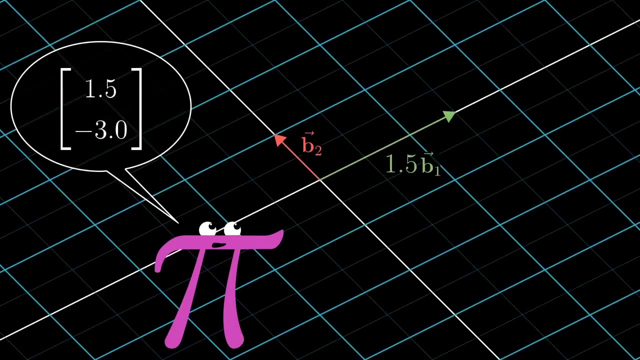 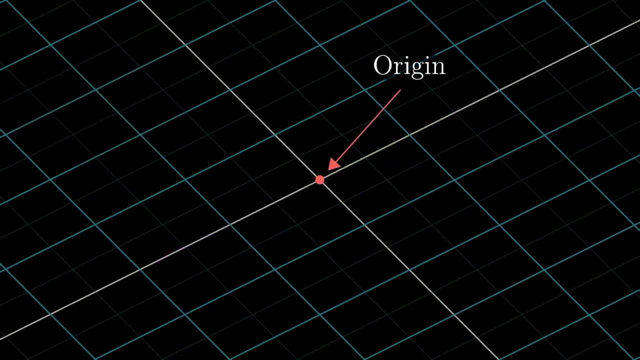 Space itself has no intrinsic grid. Jennifer might draw her own grid, which would be an equally made-up construct, meant as nothing more than a visual tool to help follow the meaning of her coordinates. Her origin, though, would actually line up with ours, since everybody. 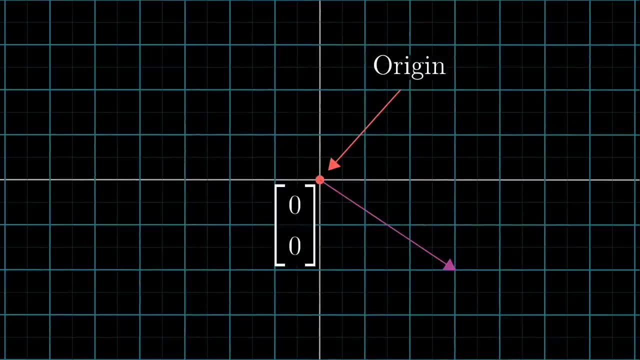 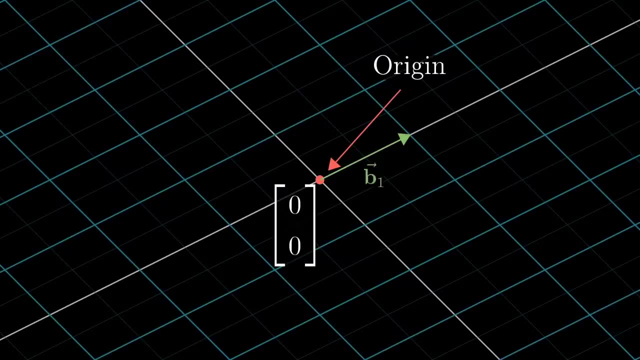 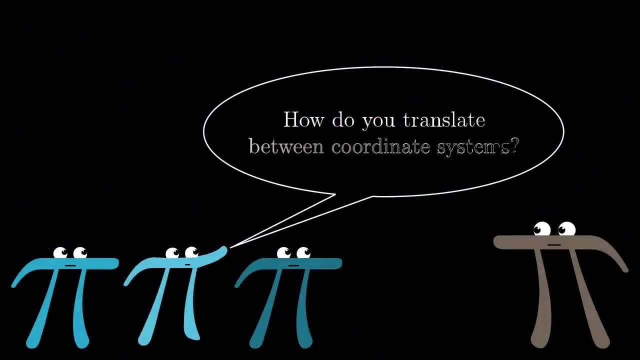 agrees on what the coordinates should mean. It's the thing that you get when you scale any vector by zero, But the direction of her axes and the spacing of her grid lines will be different depending on her choice of basis vectors. So, after all, this is set up. a pretty natural question to ask is how we translate between: 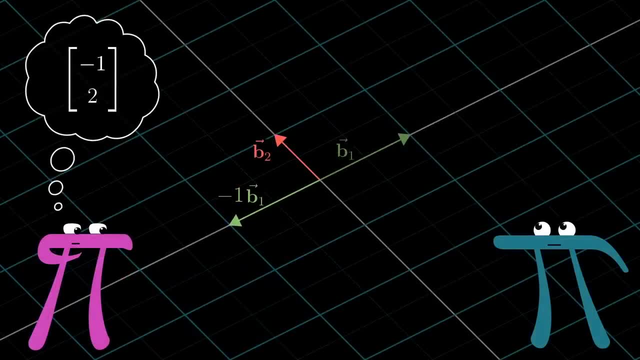 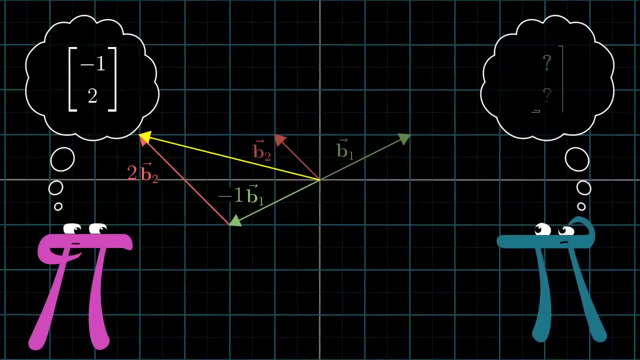 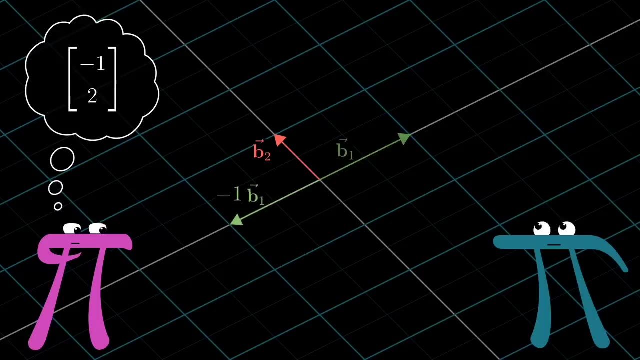 coordinate systems. If, for example, Jennifer describes a vector with coordinates, what would that be in our coordinate system? How do you translate that? Well, if you're looking at a vector with coordinates, how do you translate from her language to ours? Well, what her coordinates are saying is that this vector is negative 1 times b1. 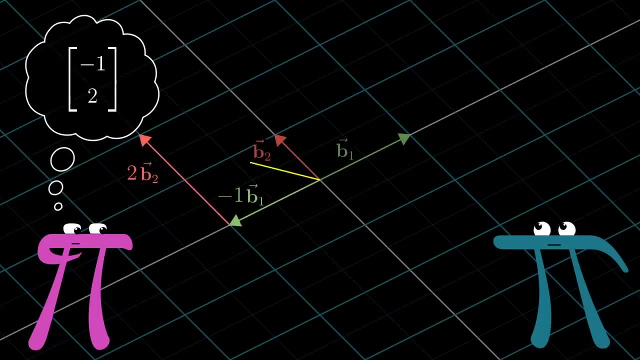 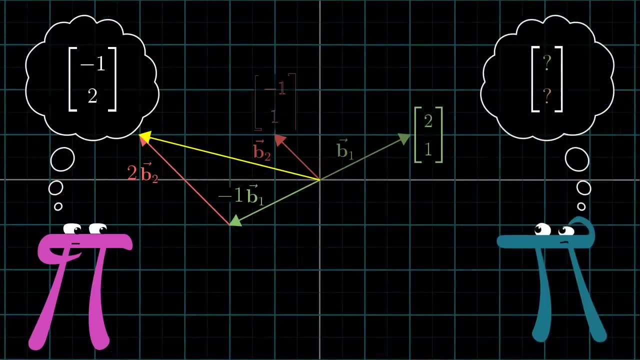 plus 2 times b2.. And from our perspective, b1 has coordinates and b2 has coordinates, So we can actually compute negative 1 times b1 plus 2 times b2 as they're represented in our coordinate system, And working this out you get a vector with coordinates. 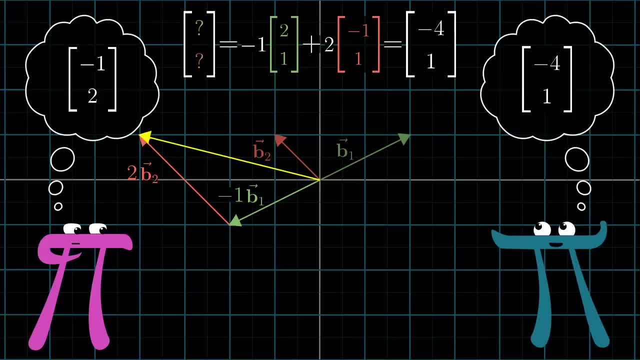 So that's how we would describe the vector that she thinks of. as This process here of scaling each of her basis vectors by the corresponding coordinates of some vector, then adding them together might feel somewhat familiar. It's matrix vector multiplication with a matrix whose columns represent Jennifer's basis vectors. 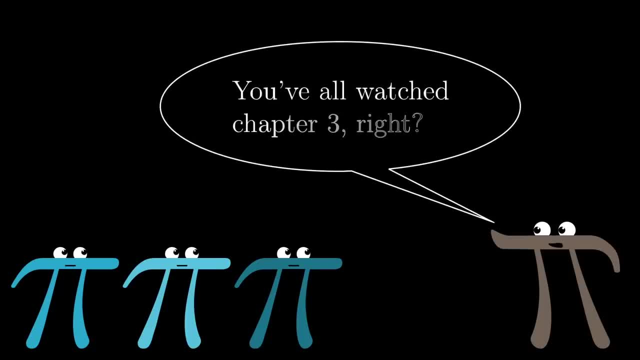 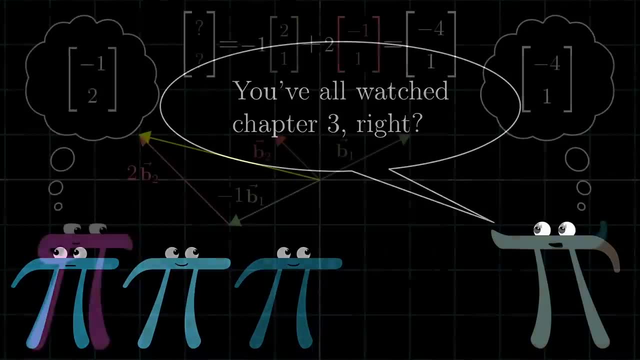 in our language. Once you understand matrix vector multiplication as applying a certain linear transformation, say by watching what I view to be the most important video in this series, chapter 3,, there's a pretty intuitive way to think about what's going on here. A matrix whose columns 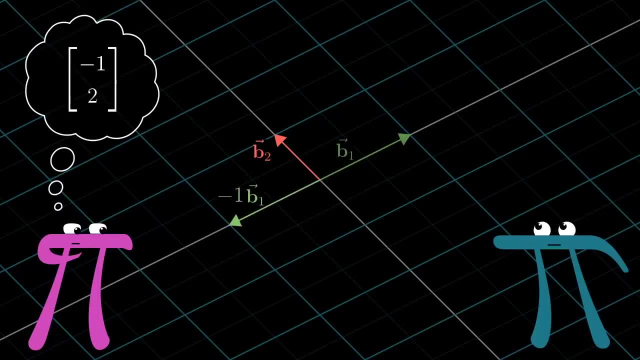 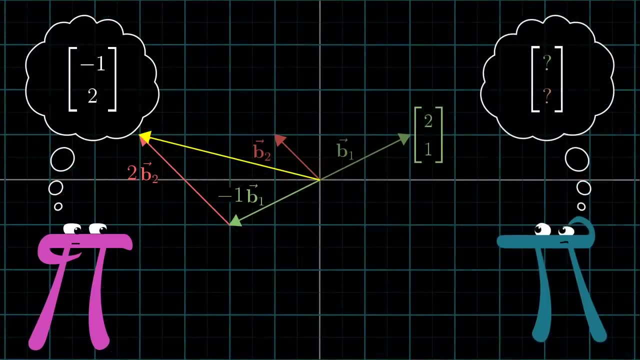 are saying is that this vector is negative 1 times b1 plus 2 times b2.. And from our perspective, b1 has coordinates and b2 has coordinates, So we can actually compute negative 1 times b1 plus 2 times b2 as they're represented in. 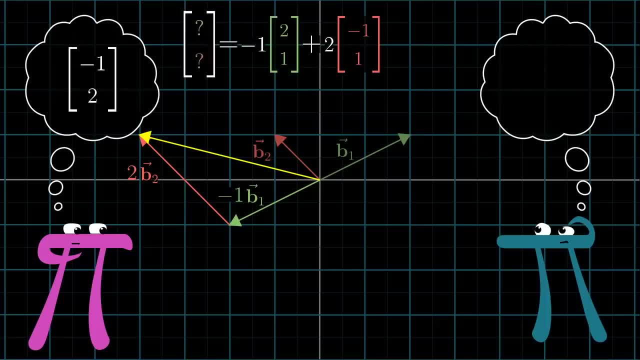 our coordinate system And working this out, you get a vector with coordinates. So that's how we would describe the vector that she thinks of- as negative 1, 2. This process here of scaling each of her basis vectors by the corresponding coordinates of 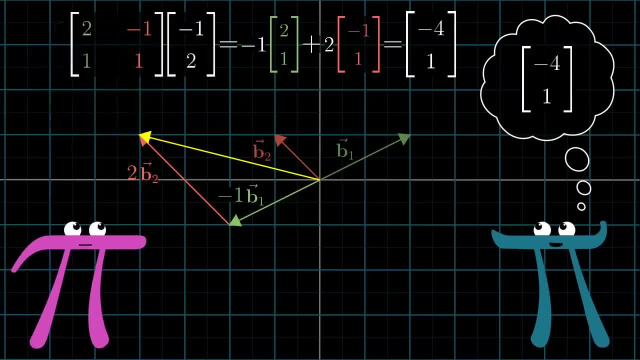 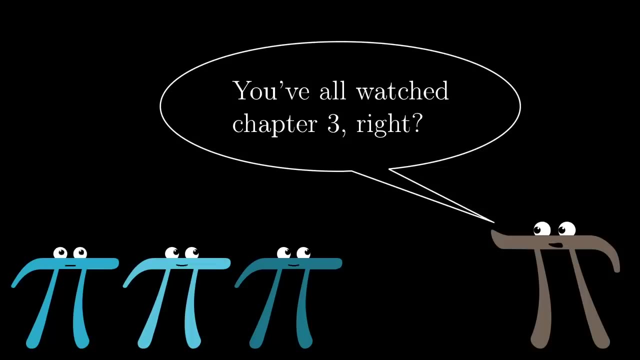 some vector, then adding them together might feel somewhat familiar. It's matrix vector multiplication, with a matrix whose columns represent Jennifer's basis vectors in our language. Now, once you understand matrix vector multiplication as applying a certain linear transformation, say by watching what I view to be the most important video in this series, chapter 3,. 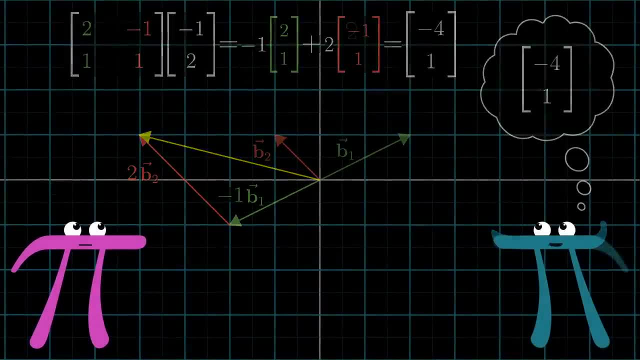 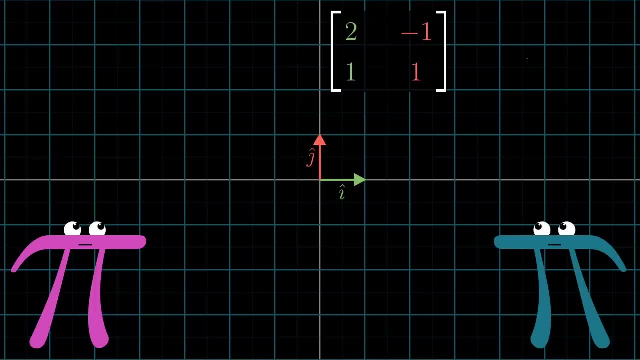 there's a pretty intuitive way to think about what's going on here. A matrix whose columns represent Jennifer's basis vectors can be thought of as a transformation that moves our basis vectors. i-hat and j-hat the things we think of when we say 1, 0 and 0, 1, to. 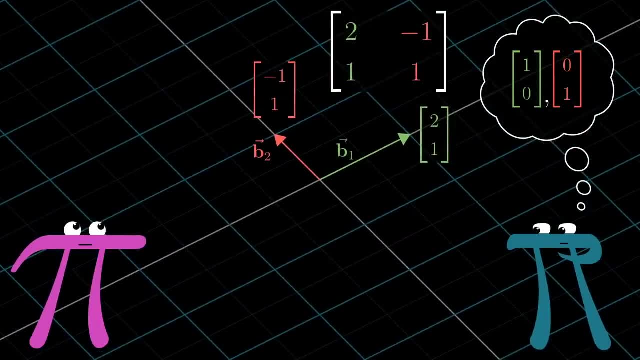 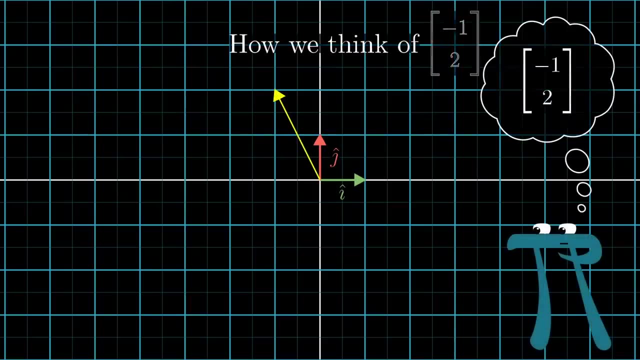 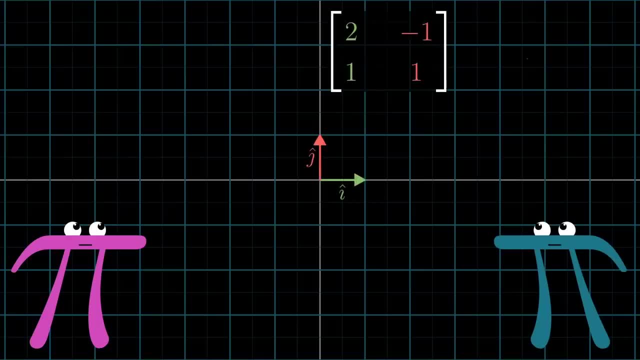 represent Jennifer's basis vectors can be thought of as a transformation that moves our basis vectors, i-hat and j-hat. the things we think of when we say 1, 0, and 0, 1, to Jennifer's basis vectors. the things she thinks of when she says 1, 0, and 1, 0, and 1, 0,. 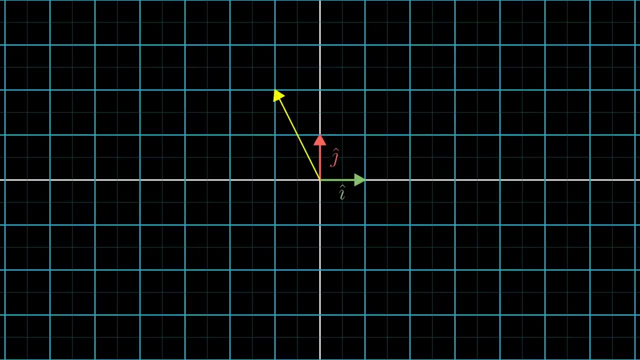 and 0, and 0, 1.. To show how this works, let's walk through what it would mean to take the vector that we think of as having coordinates and applying that transformation Before the linear transformation. we're thinking of this vector as a certain linear combination. 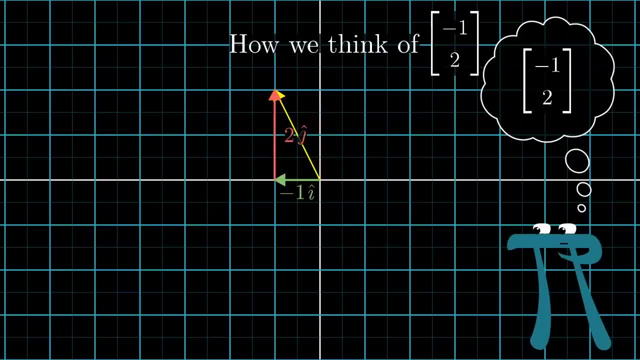 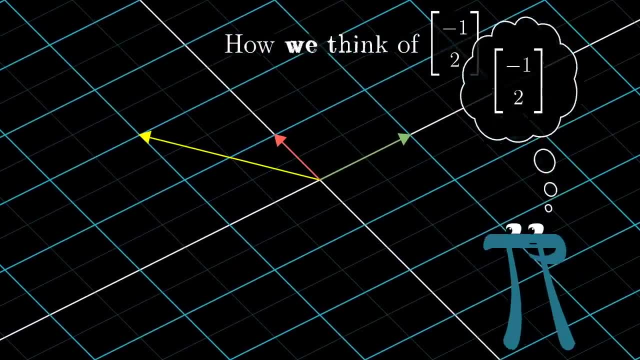 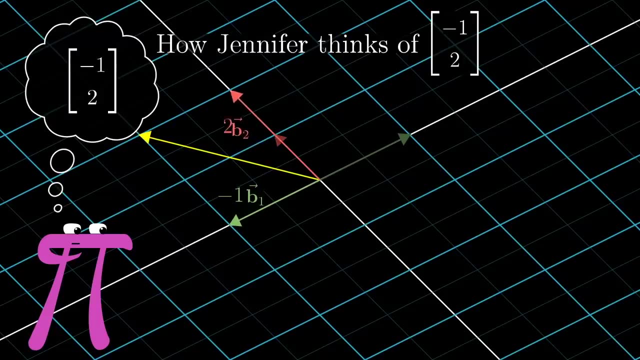 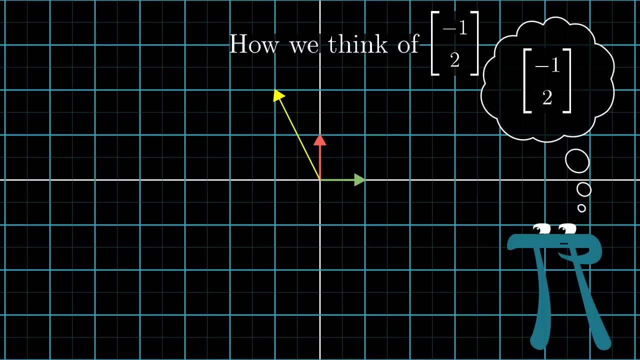 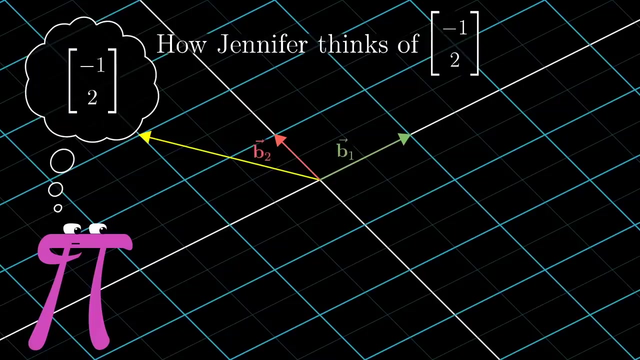 of our basis vectors, And the key feature of a linear transformation is that the resulting vector will be that same linear combination, but of the new basis vectors. So what this matrix does is transform our misconception of what Jennifer means into the actual vector that she's referring to. 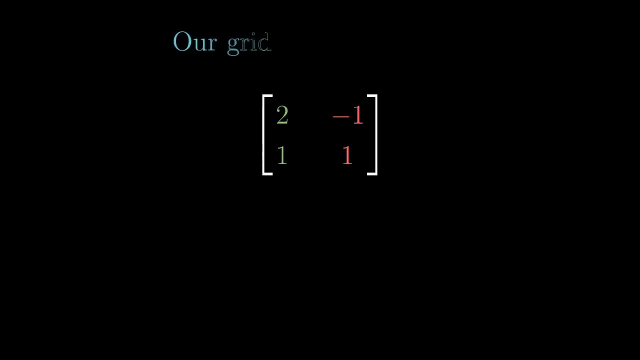 I remember that when I was first learning this it always felt kind of backwards to me. Geometrically, this matrix transforms our grid into Jennifer's grid, but numerically it's translating a vector described in her language into Jennifer's grid. 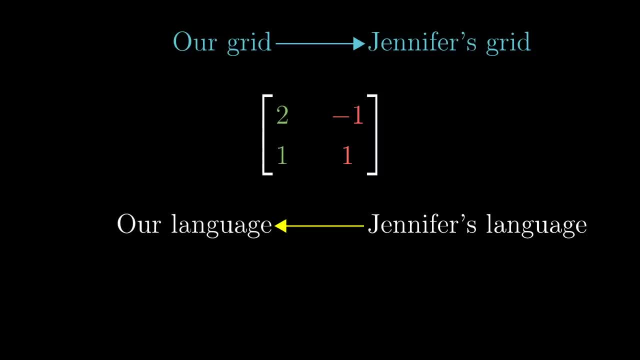 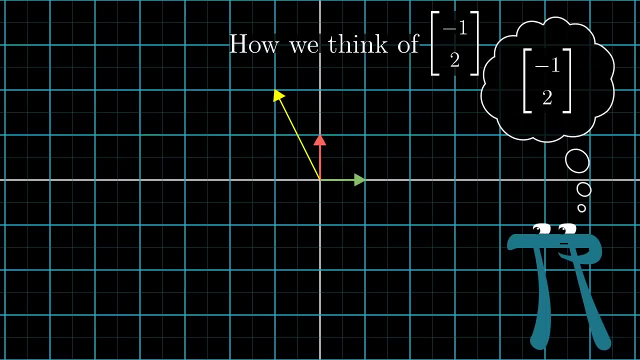 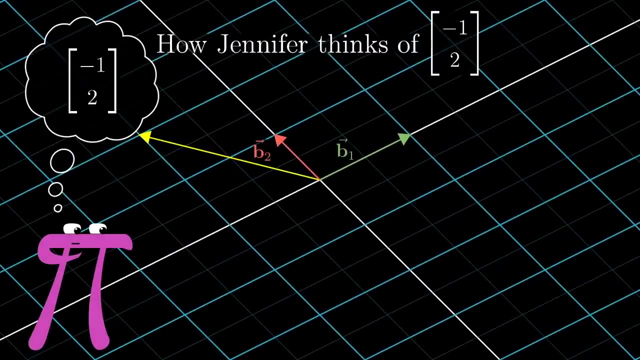 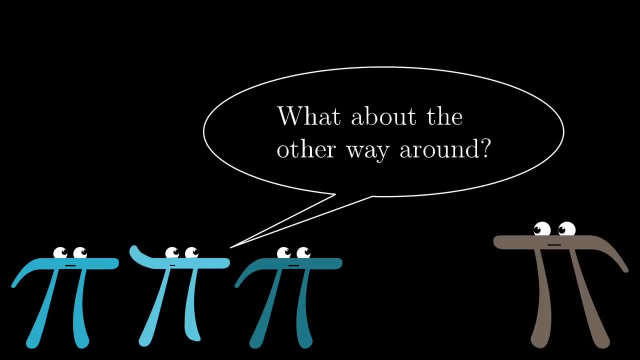 What made it finally click for me was thinking about how it takes our misconception of what Jennifer means: the vector we get using the same coordinates, but in our system then it transforms it into the vector that she really meant. What about going the other way around? In the example I used earlier this video when 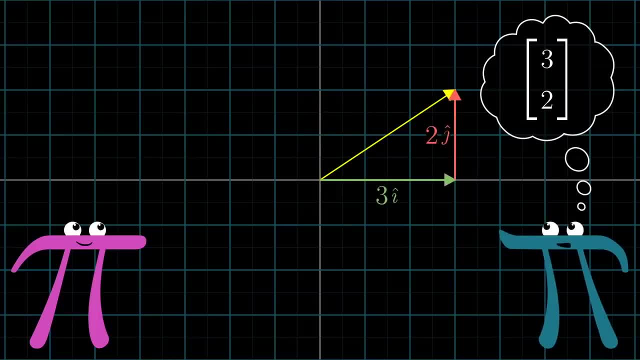 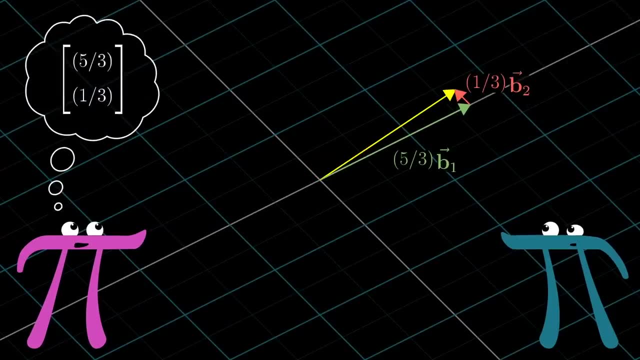 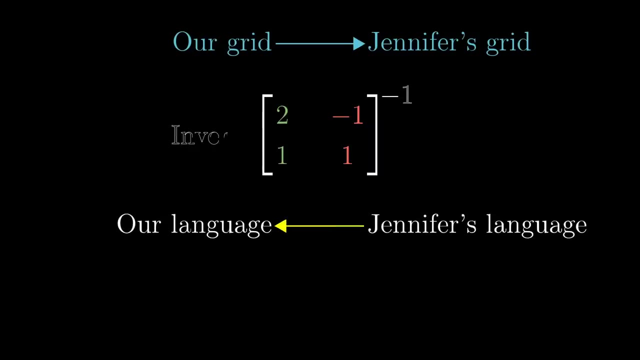 I had the vector with coordinates in our system. how did I compute that it would have coordinates 5 thirds and 1 third in Jennifer's system? You start with that change of basis matrix that translates Jennifer's language into ours. then you take its inverse. 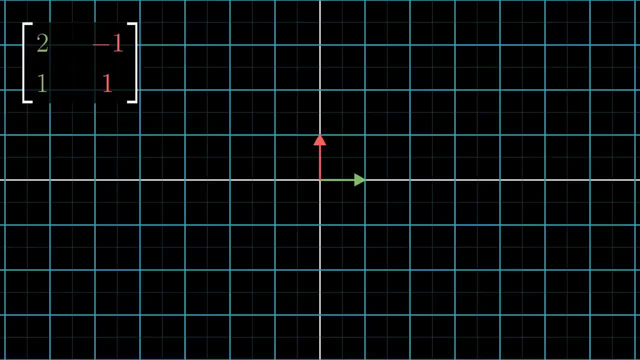 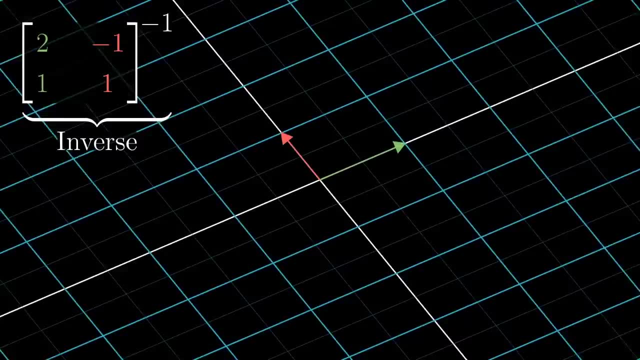 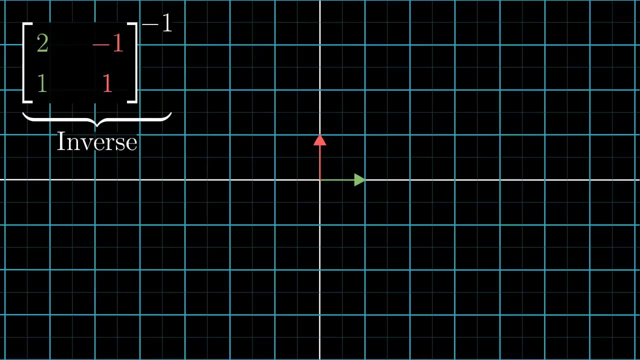 Remember, the inverse of a transformation is a new transformation. that corresponds to playing that first one backwards. In practice, especially when you're working in more than two dimensions, you'd use a computer to compute the matrix that actually represents this inverse, In this case the inverse of the change of basis matrix that has Jennifer's basis as: 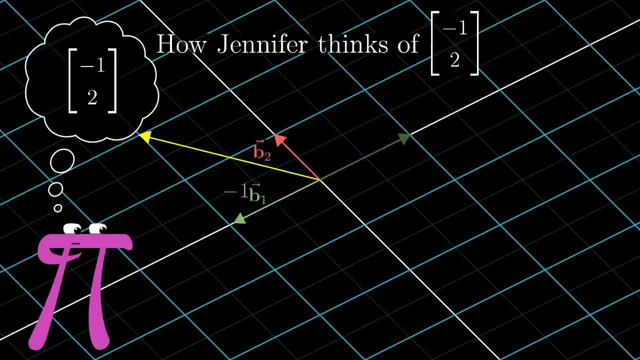 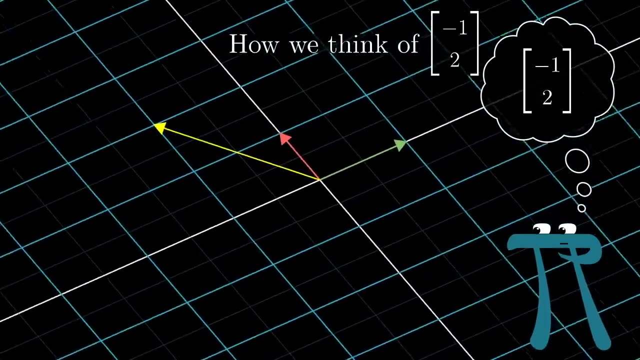 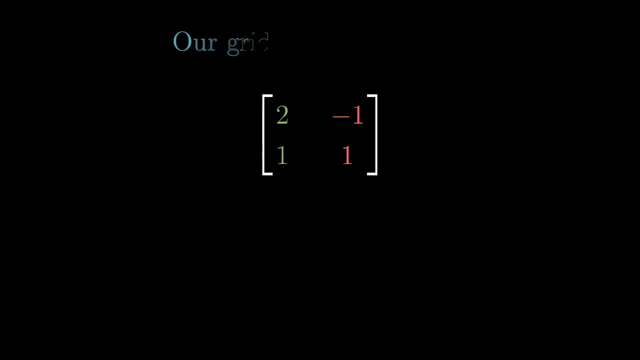 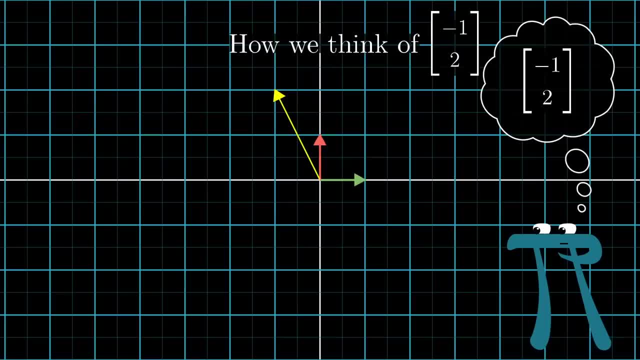 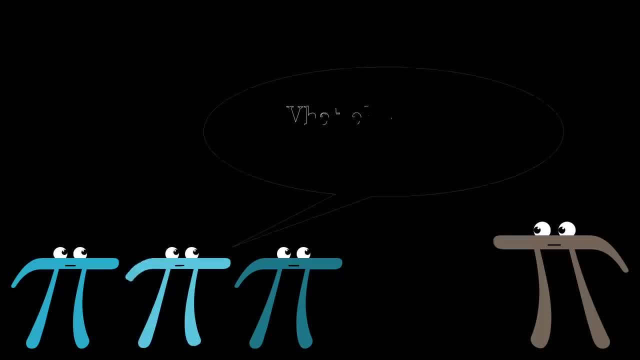 of what Jennifer means: the vector we get using the same coordinates, but in our system then it transforms it into the vector that she really meant. What about going the other way around? In the example I used earlier this video when I had the vector with coordinates three, two. 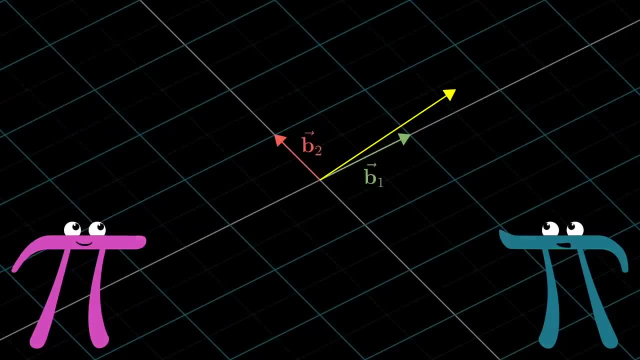 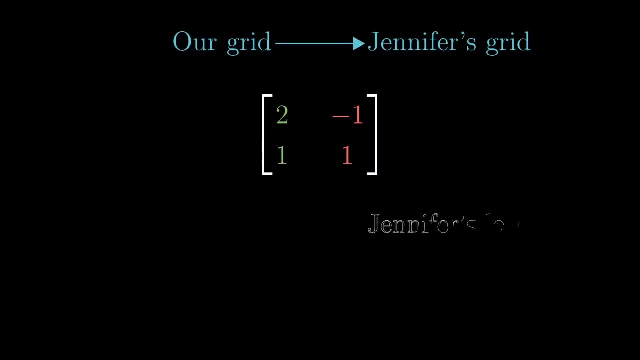 in our system. how did I compute that it would have coordinates: five thirds and one third in Jennifer's system. You start with that change of basis matrix that translates Jennifer's language into ours. then you take its inverse. Remember the inverse of a transformation. 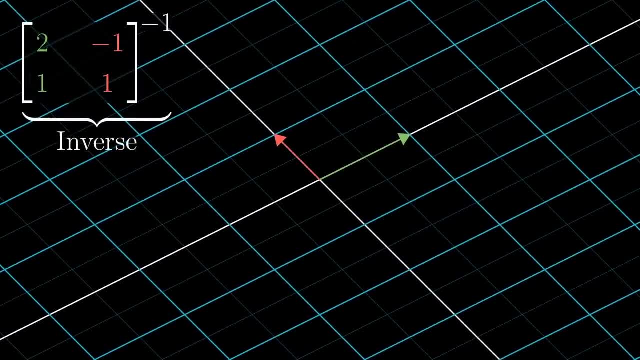 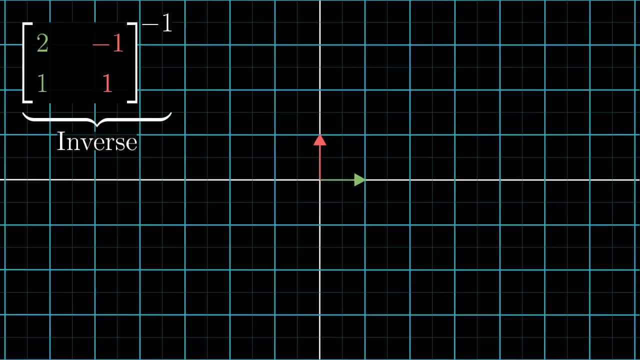 is a new transformation that corresponds to playing that first one backwards. In practice, especially when you're working in more than two dimensions, you'd use a computer to compute the matrix that actually represents this inverse, In this case the inverse of the change of basis matrix. 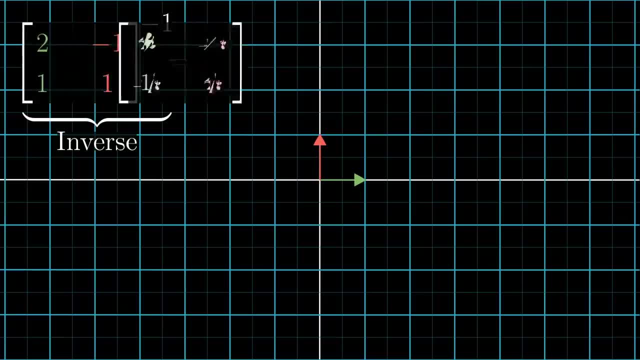 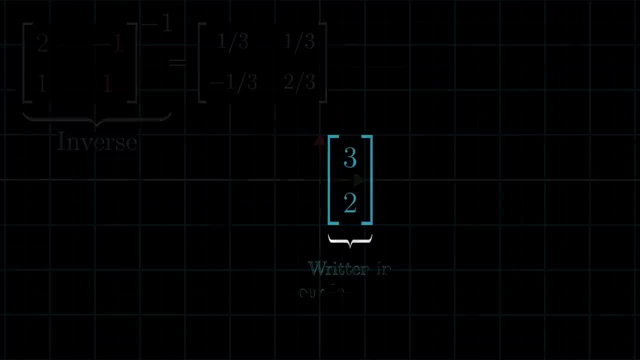 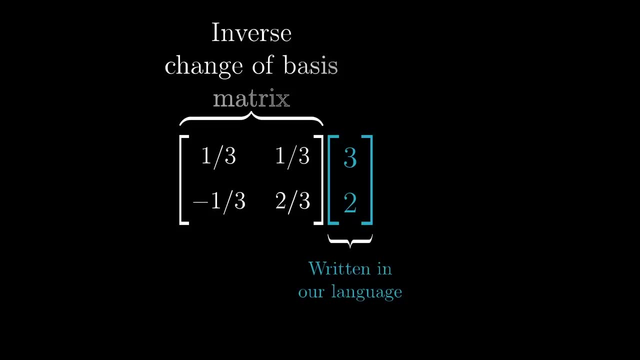 that has Jennifer's basis as its columns ends up working out to have columns one third negative one third and one third two thirds. So for example, to see what the vector three two looks like in Jennifer's system, we multiply this inverse change of basis matrix. 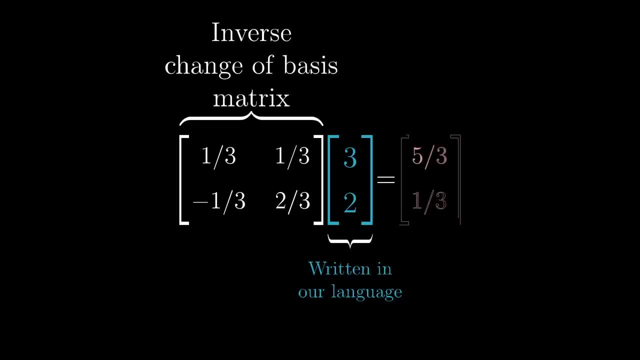 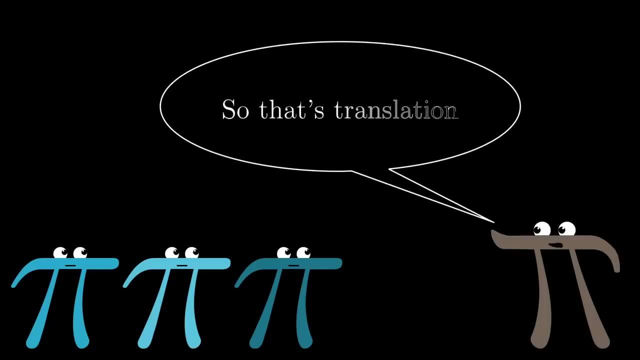 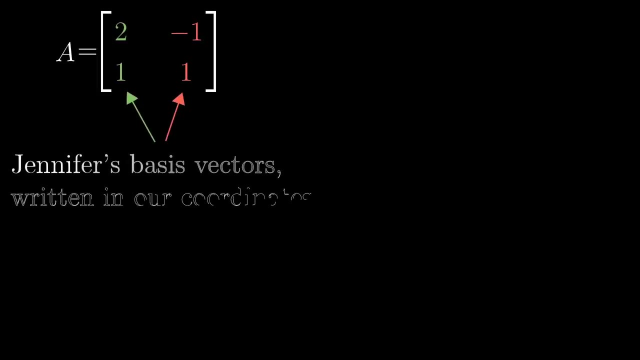 by the vector three, two which works out to be five thirds, one third. So that, in a nutshell, is how to translate the description of individual vectors back and forth between coordinate systems. The matrix whose columns represent Jennifer's basis: vectors. 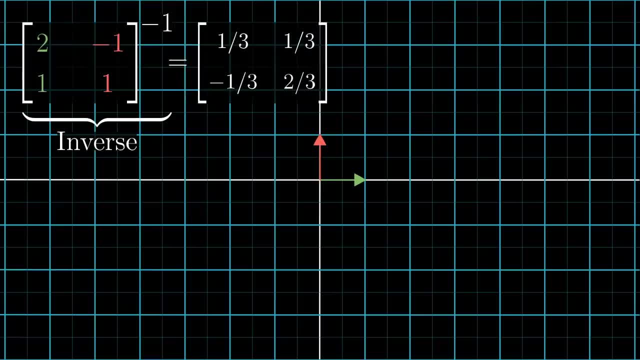 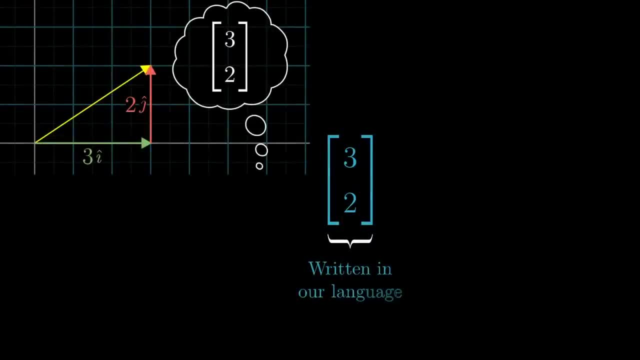 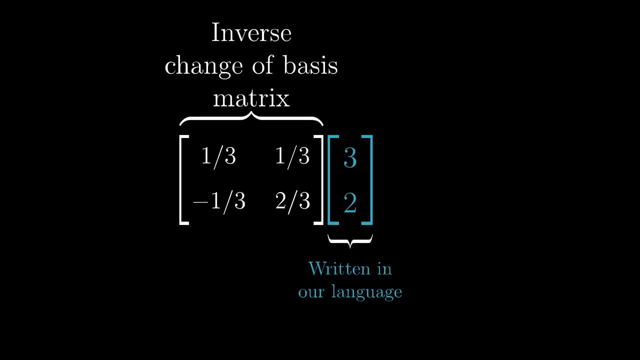 its columns ends up working out to have columns 1 third negative, 1 third and 1 third, 2 thirds. So, for example, to see what the vector 3: 2 looks like in Jennifer's system, we multiply this inverse change of basis matrix by the vector 3- 2, which works out to be 5 thirds. 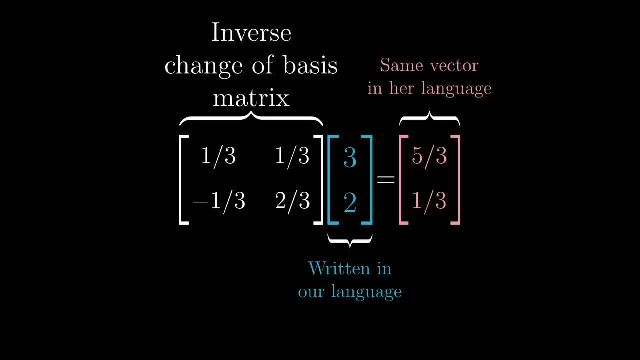 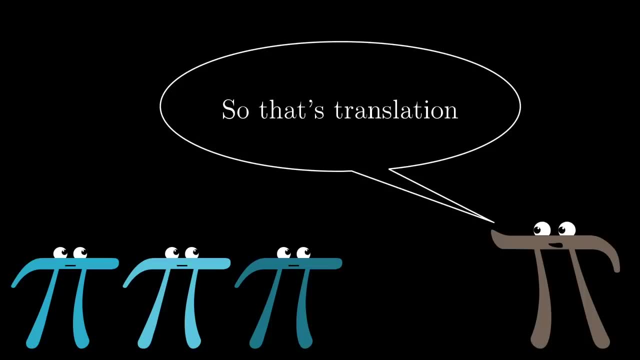 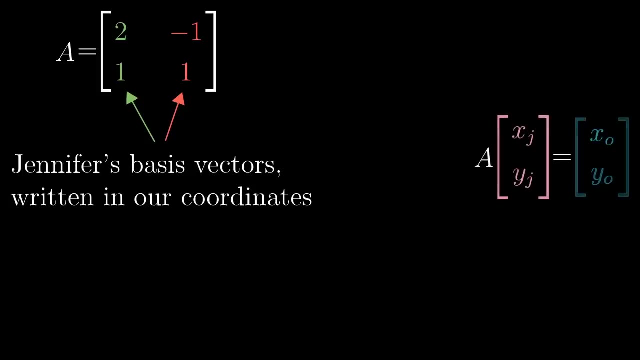 1. third. So that, in a nutshell, is how to translate the description of individual vectors back and forth between coordinate systems. The matrix, whose columns represent Jennifer's basis vectors but written in our coordinates, translates vectors from her language into our language, And the inverse matrix does the opposite. 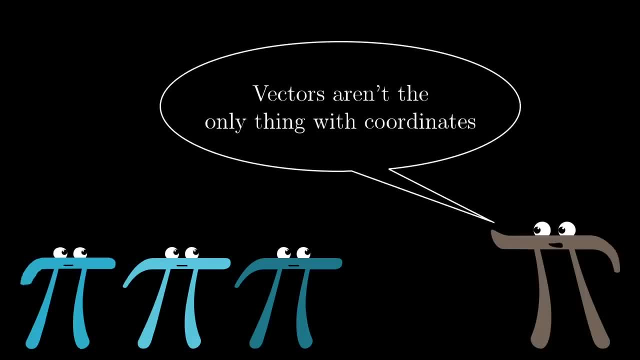 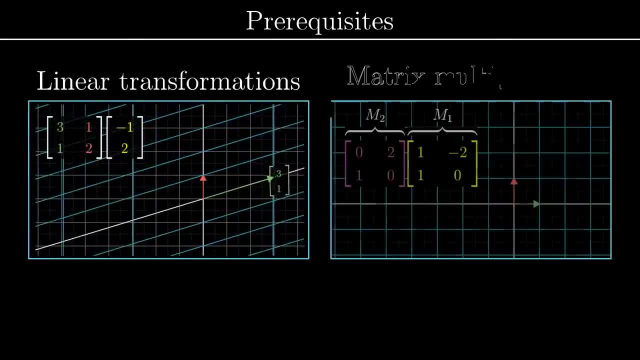 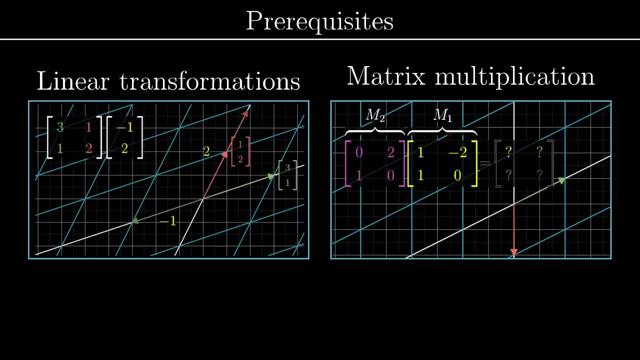 But vectors aren't the only thing that we describe using coordinates. For this next part, it's important that you're all comfortable representing transformations with matrices and that you know how matrix multiplication corresponds to composing successive transformations. Definitely pause and take a look at chapters 3 and 4 if any of that feels uneasy. 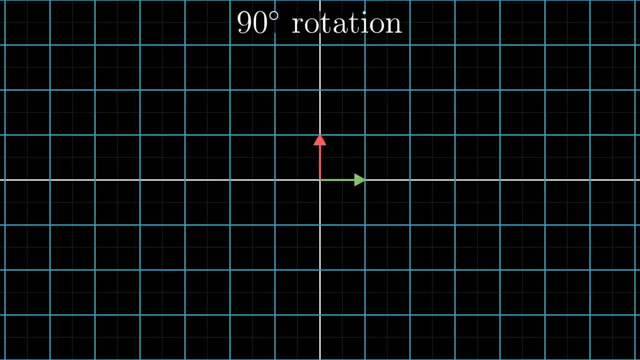 Consider some linear transformation like a 90 degree counterclockwise rotation. When you and I represent this with a matrix, we follow where the basis vectors i-hat and j-hat each go: i-hat ends up at the spot with coordinates and j-hat ends up at the spot with coordinates. 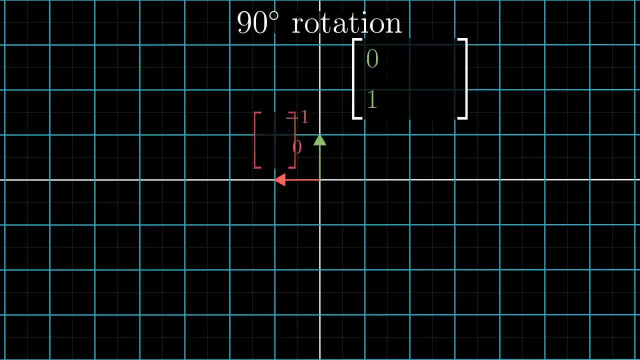 So those coordinates become the columns of our matrix. But this representation is heavily tied up in our choice of basis vectors, from the fact that we're following i-hat and j-hat in the first place to the fact that we're recording their landing spots in our own coordinate system. 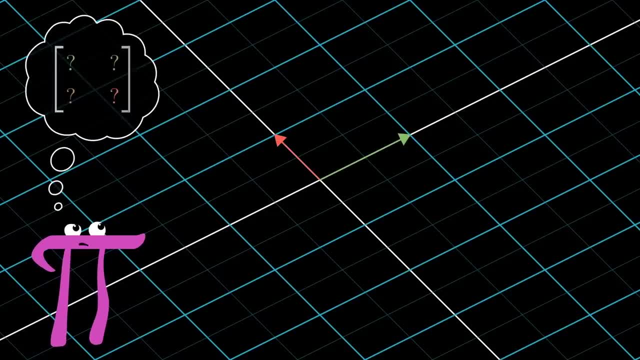 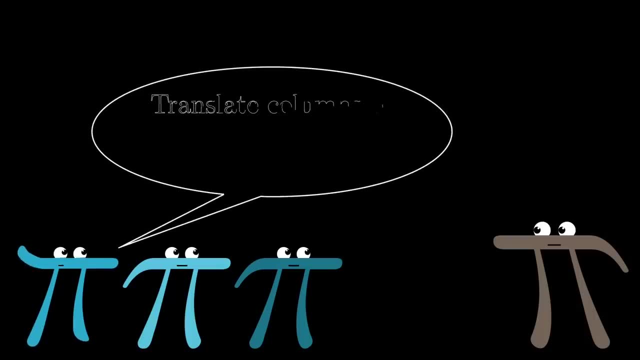 How would Jennifer describe this same 90 degree rotation of space? How would Jennifer describe this same 90 degree rotation of space? You might be tempted to just translate the columns of our rotation matrix into Jennifer's language, but that's not quite right. 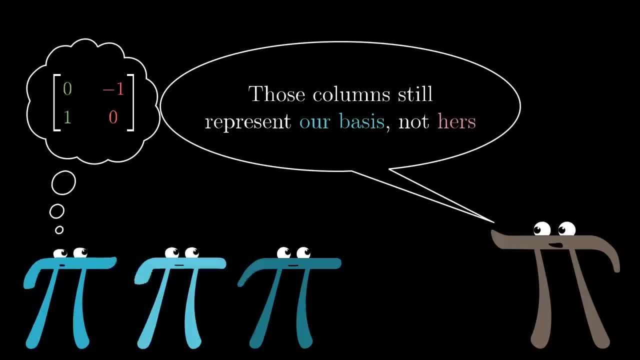 Those columns represent where our basis vectors- i-hat and j-hat- go, but the matrix that Jennifer wants should represent where her basis vectors land, and it needs to describe those landing spots in her language. Here's a common way to think of how this is done. 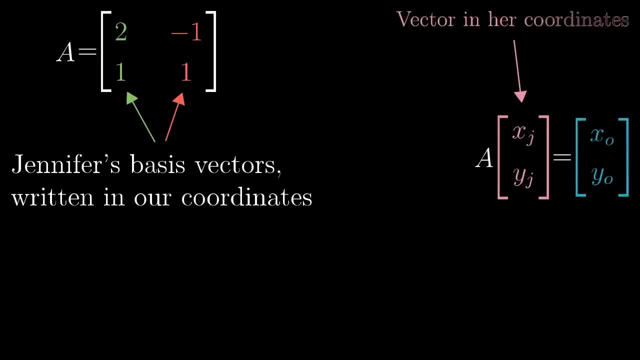 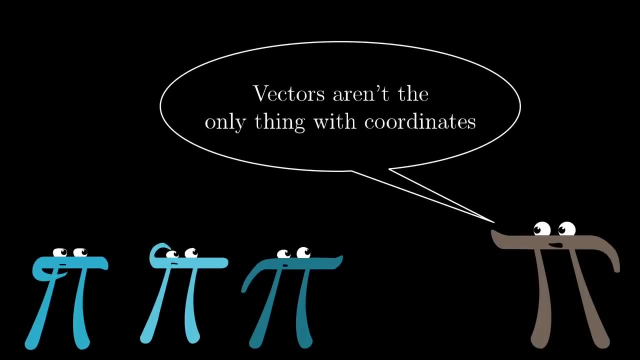 but written in our coordinates, translates vectors from her language into our language And the inverse. matrix does the opposite. But vectors aren't the only thing that we describe using coordinates. For this next part, it's important that you're all comfortable representing transformations with matrices and that you know how matrix multiplication. 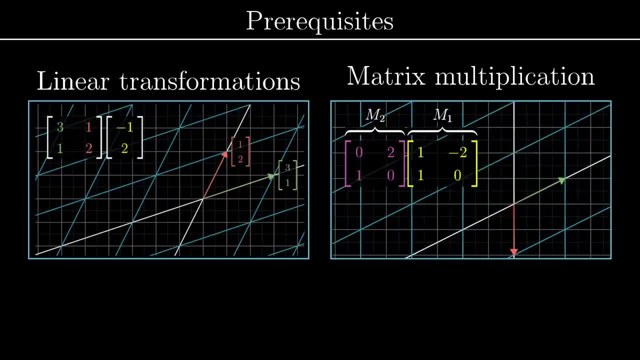 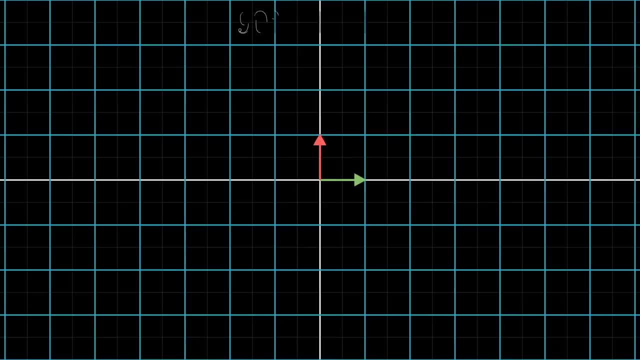 corresponds to composing successive transformations. Definitely pause and take a look at chapters three and four if any of that feels uneasy. Consider some linear transformation like a 90 degree counterclockwise rotation, When you and I represent this with a matrix, we follow where the basis vectors i-hat and j-hat each go. 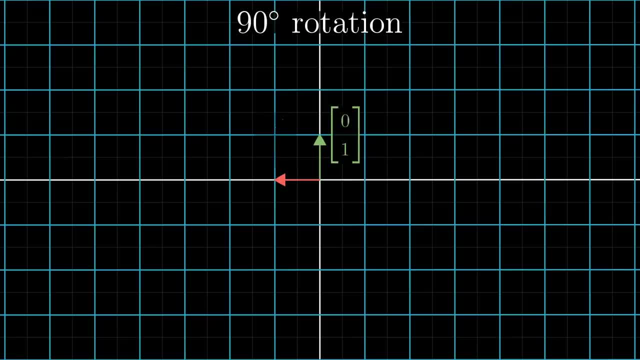 i-hat ends up at the spot with coordinates zero one, and j-hat ends up at the spot with coordinates negative one- zero. So those coordinates become the columns of our matrix. But this representation is heavily tied up in our choice of basis vectors. 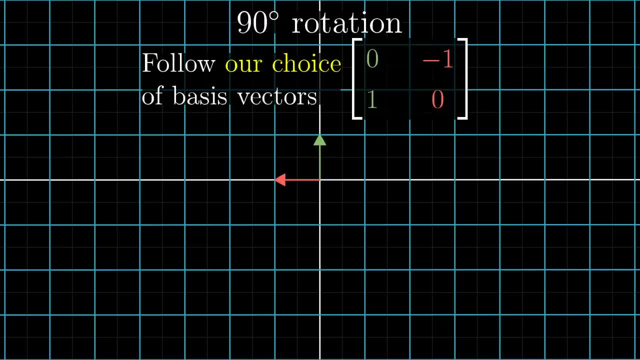 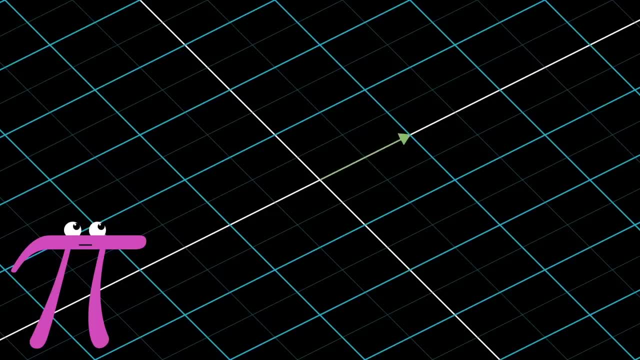 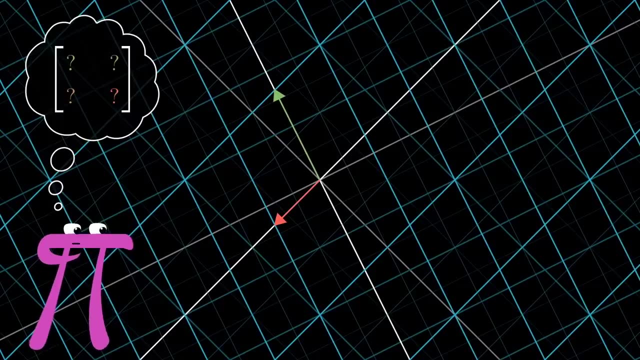 from the fact that we're following i-hat and j-hat in the first place to the fact that we're recording their landing spots in our own coordinate system. How would Jennifer describe this same 90 degree rotation of space? You might be tempted to just translate the columns. 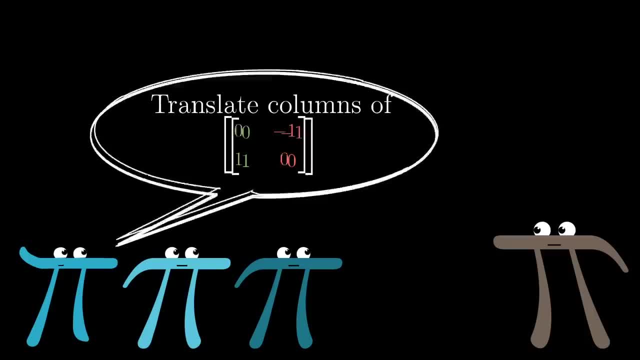 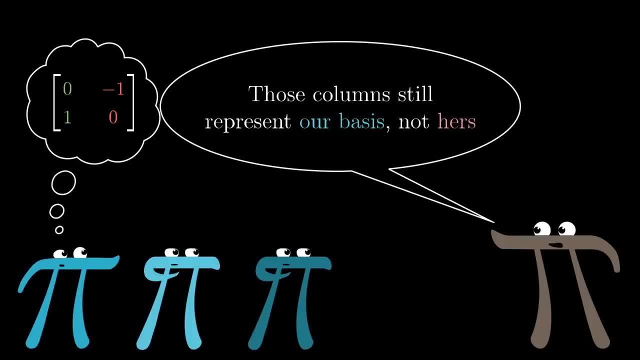 of our rotation matrix into Jennifer's language, but that's not quite right. Those columns represent where our basis vectors- i-hat and j-hat- go, but the matrix that Jennifer wants should represent where her basis vectors land and it needs to describe those landing spots. 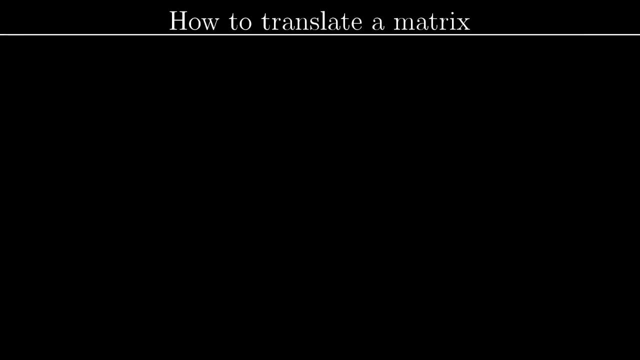 in her language. Here's a common way to think of how this is done. Start with any vector written in Jennifer's language, Rather than trying to follow what happens to it in terms of her language. first. we're gonna translate it into our language. 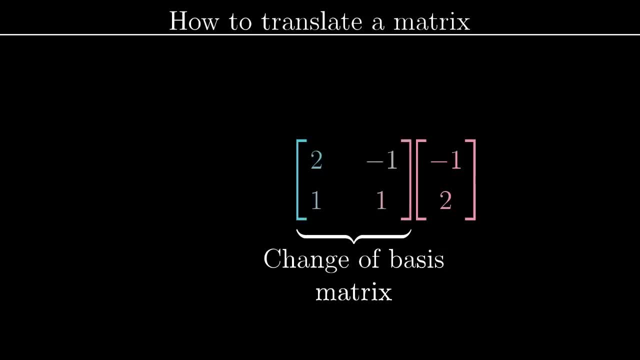 using the change of basis matrix, The one whose columns represent her basis vectors in our language. This gives us the same vector, but now written in our language. Then apply the transformation matrix to what you get by multiplying it on the left. This tells us: 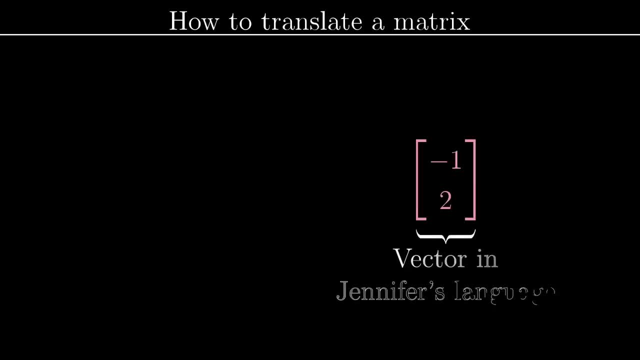 Let's start with any basis vector. Let's start with any vector written in Jennifer's language, Rather than trying to follow what happens to it in terms of her language. first, we're going to translate it into our language using the change of basis matrix, the one whose 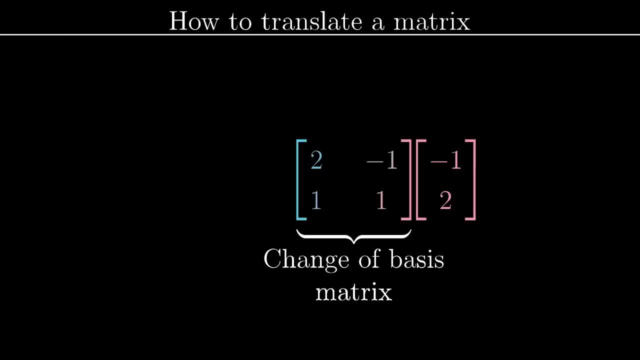 columns represent her basis vectors in our language. This gives us the same vector, but now written in our language. Then apply the transformation matrix to what you get by multiplying it on the left. This tells us where that vector lands, but still in our language. 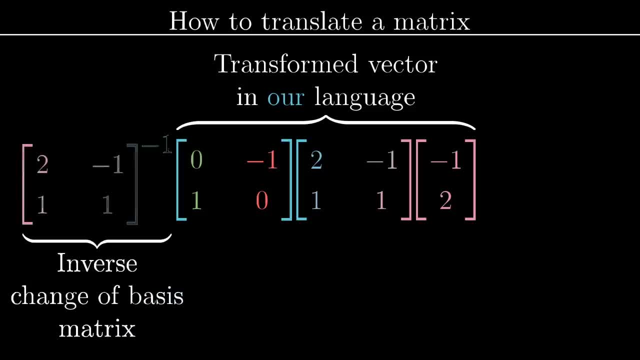 So let's start with any vector written in Jennifer's language. So, as a last step, apply the inverse change of basis matrix multiplied on the left, as usual, to get the transformed vector, but now in Jennifer's language, Since we could do this with any vector written in her language. first applying the change, 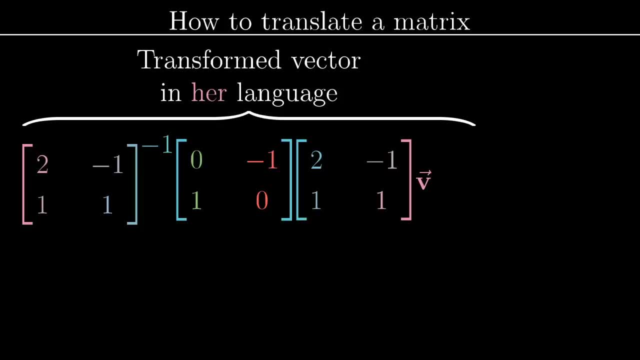 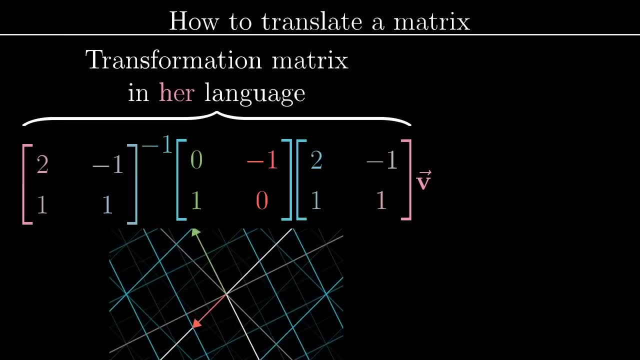 of basis, then the transformation, then the inverse change of basis. that composition of three matrices gives us the transformation matrix in Jennifer's language. It takes in a vector of her language and spits out the transformed vector. but now in Jennifer's language. 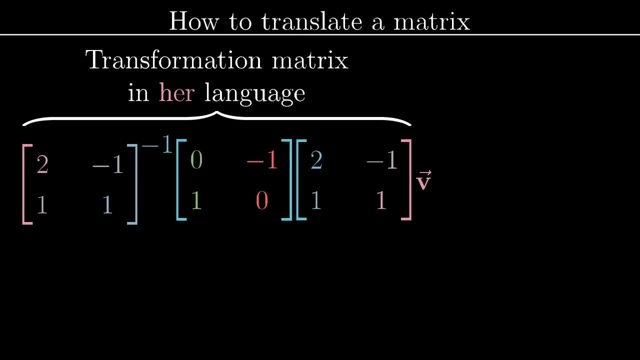 So now we have the transformation matrix in Jennifer's language. Let's look at the transformation matrix in Jennifer's language For this specific example. when Jennifer's basis vectors look like 2,1 and negative 1,1 in our language, and when the transformation is a 90 degree rotation, the product of these 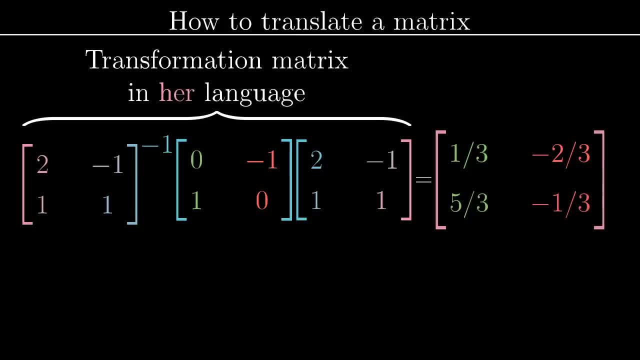 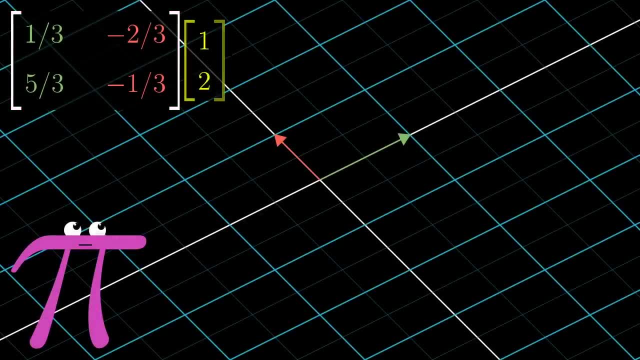 three matrices. if you work through it has columns 1,3,5, and negative 2,3,, negative 1,3. So if Jennifer multiplies that matrix by the coordinates of a vector in her system, it will return the 90-degree rotated version of that vector in her language. 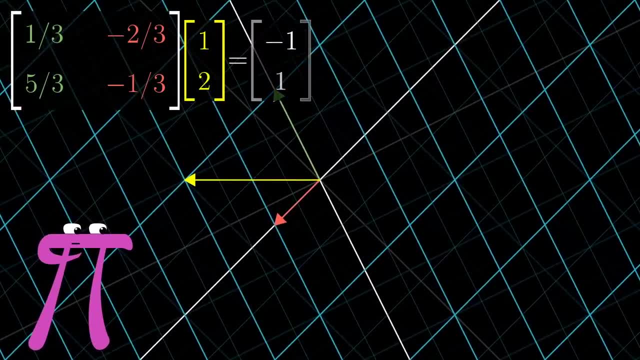 So if Jennifer multiplies that matrix by the coordinates of a vector in her system, it will return the 90-degree rotated version of that vector in her language. So if the transformation matrix in Jennifer's language does not correspond to the transformation matrix in her language and if it does not correspond to the transformation matrix in 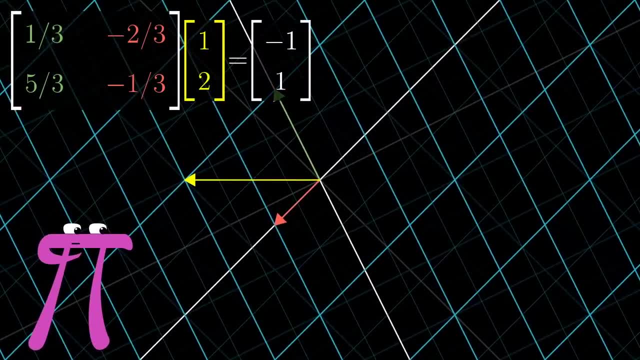 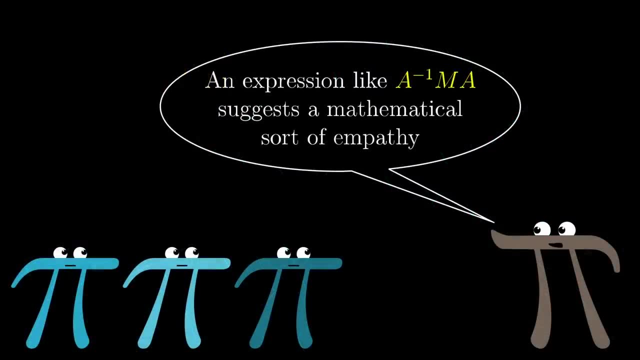 her language, it will return the 90-degree rotated version of that vector expressed in her coordinate system. In general, whenever you see an expression like a inverse times m, times a, it suggests a mathematical sort of empathy. That middle matrix represents a transformation of some kind. as you see it, 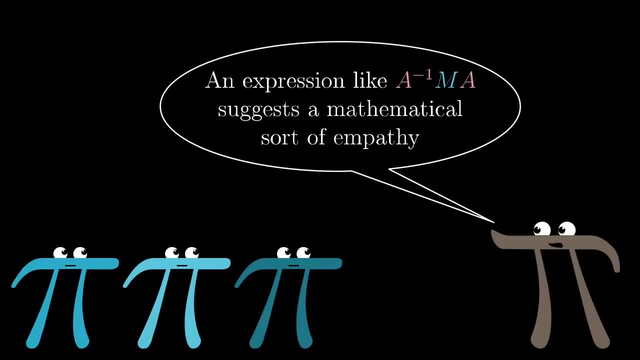 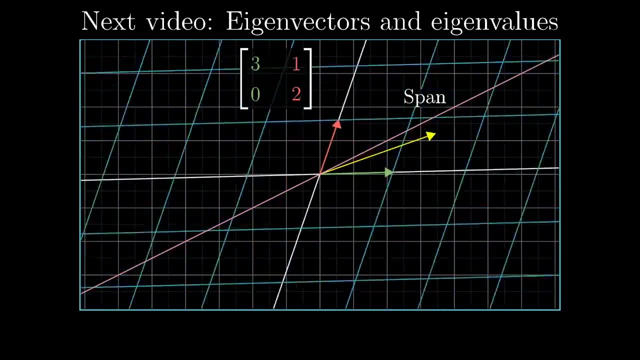 And the outer two matrices represent the empathy, the shift in perspective, And the full matrix product represents that same transformation, but as someone else sees it. For those of you wondering why we care about alternate coordinate systems, the next video on eigenvectors and eigenvalues will give a really important example of this. See you then.